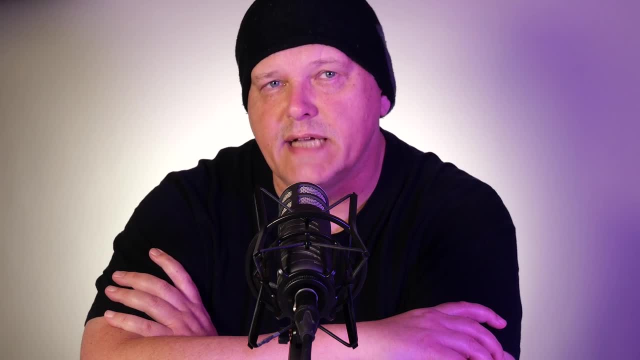 of the SQL language. However, to be compliant with the ANSI standard, they all have to support at least the major commands such as select, update, delete and insert, All in a similar manner. If you've heard someone say SQL is just SQL, that's what they mean. However, there's a caveat. 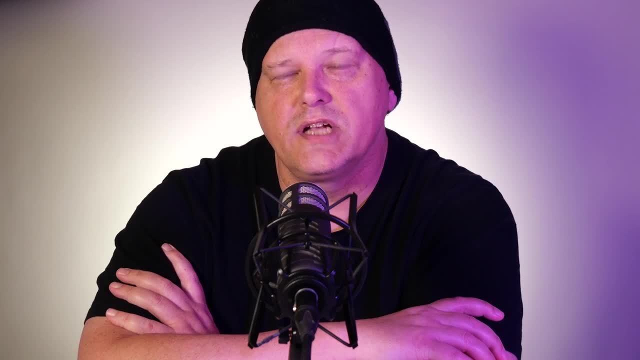 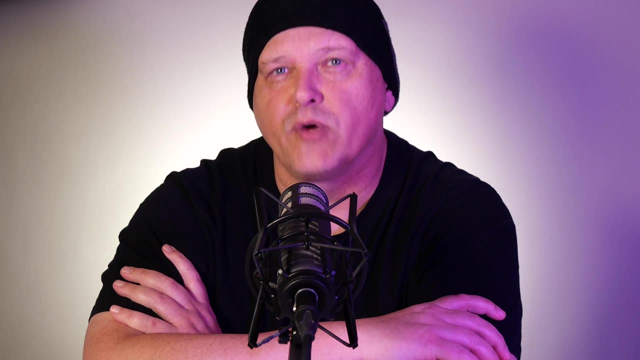 here, and it's a big one. All vendors that adopt SQL change it or tweak it a little. That means all vendors have their own flavor of SQL. For example, SQL Server's flavor of SQL is called Transact SQL. Oracle's flavor is called PLSQL. Snowflake's flavor is called SnowSQL, The SQL 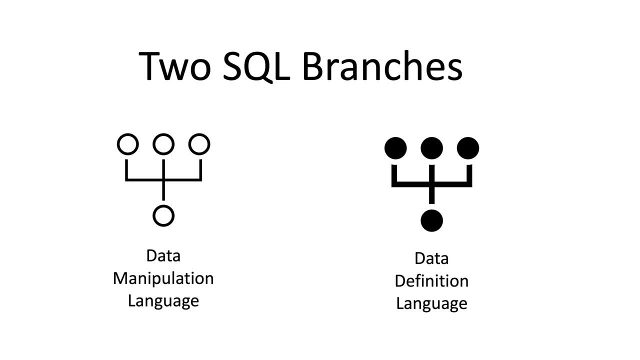 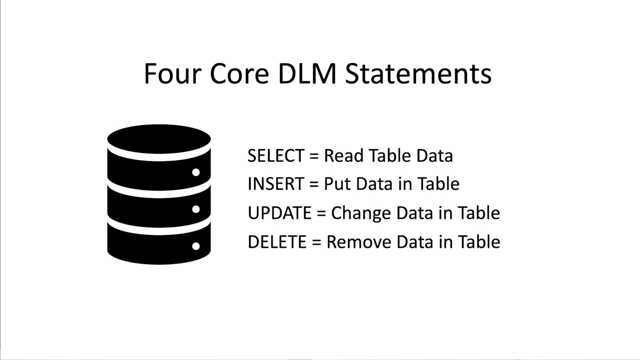 language is broken into two major branches. The first branch is DML. DML is an acronym that stands for Data Manipulation Language. DDL is an acronym that stands for Data Definition Language. DML is used to work with data in tables. There are four core DML statements. They are select: 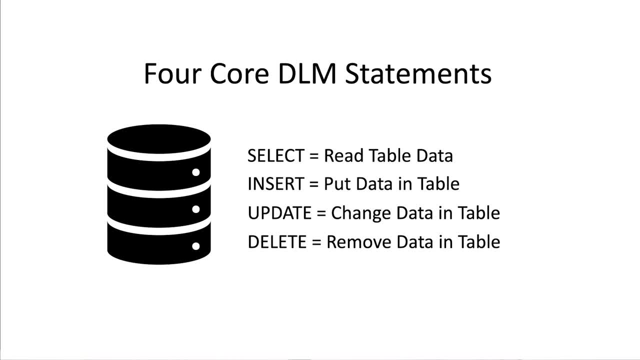 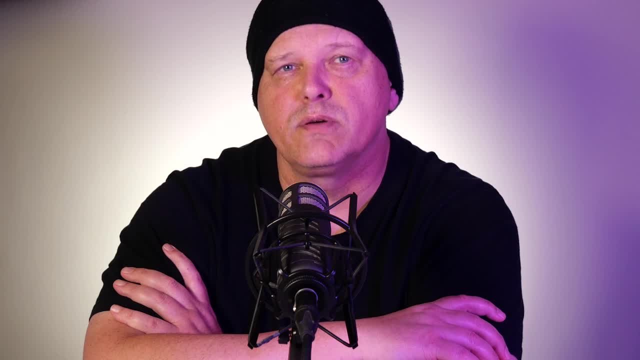 insert, update and delete. Select means to read the data in the table. Insert means to put the data in that table. Update means to change the data in that table And then delete means to remove the data in that table. Data analysts and SQL developers spend most of the time on the DML. 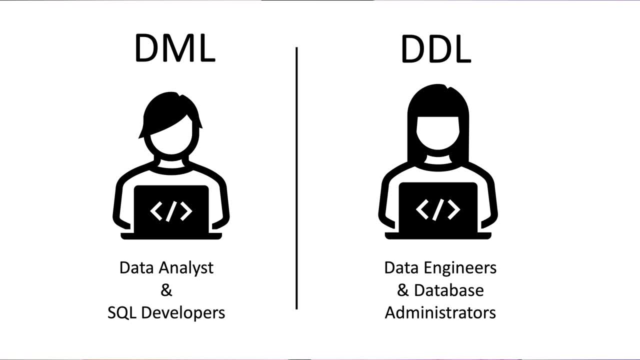 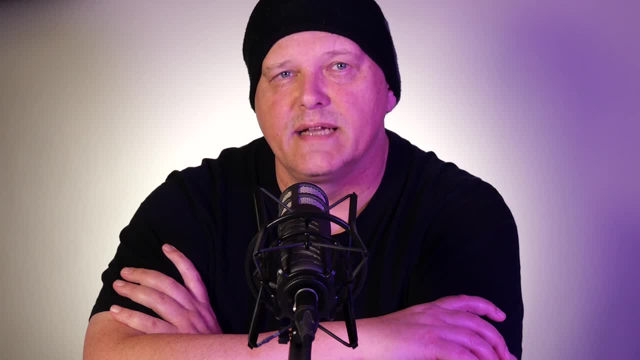 site DML is used to read the data in the table. Insert means to put the data in the table Update of the house, while DBAs and data engineers spend most of their time in the DDL side of the house. Why is that? Data analysts author SQL code that manipulates the data in the tables. 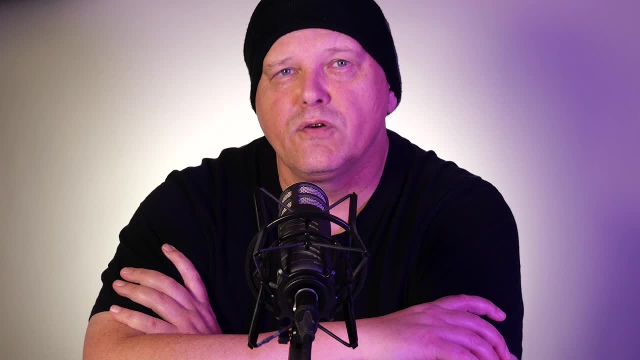 The majority of this manipulation is reading the data. If you're creating a dashboard or a KPI, then you only need to author SELECT statements. A SELECT statement returns data. If you're reading data, think SELECT. DBAs and data engineers are often responsible for creating the objects. 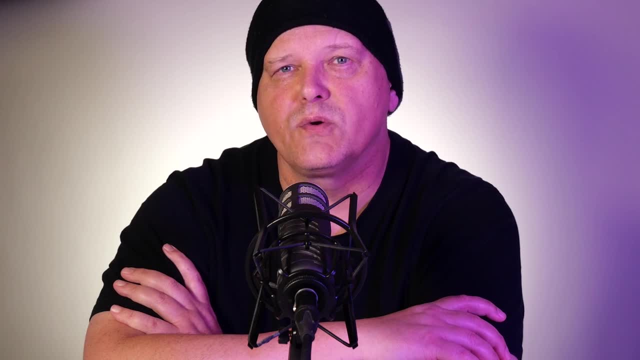 to store the data. An example of a DDL statement is the CREATE TABLE statement. Before you can insert data into a table, you first need to create the table. In most sql flavors, in order to create a table, you issue the CREATE TABLE statement. 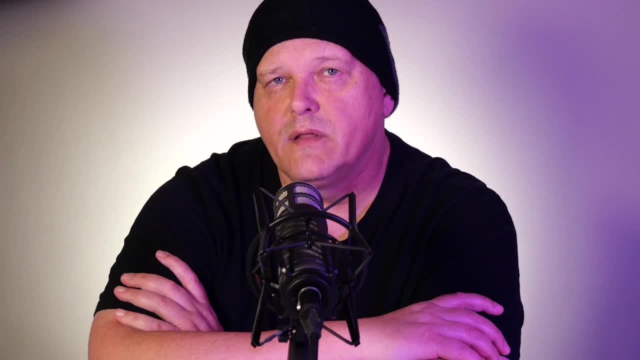 As the data engineer, I'm going to create the destination tables that are going to house the data from the relational database. Those tables have to be created before you can create a pipeline and move data to it. The creation of the tables, the pipeline and all the other structures required for 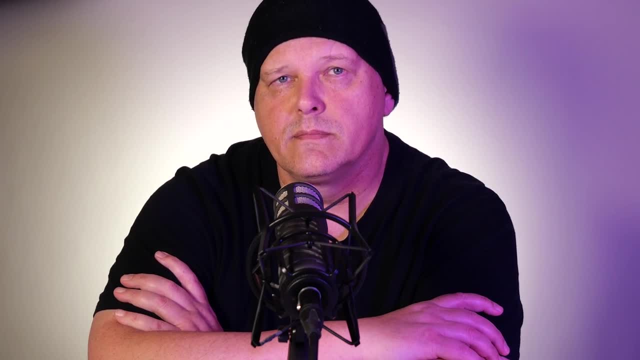 DDA are driven by different systems of information. they don't need to go approving a table. data movement is the responsibility of the data engineer. All those structures are created using DDL. If you're just starting out learning SQL, keep this separation in mind. If you're massaging, 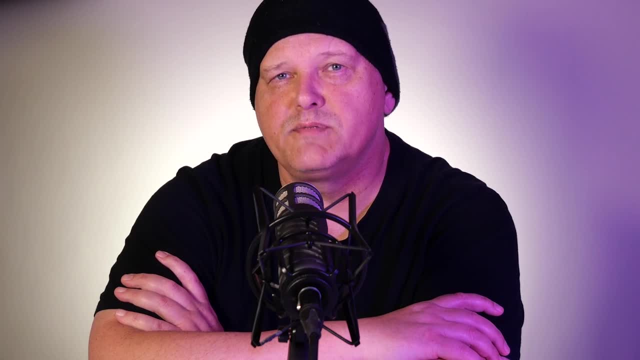 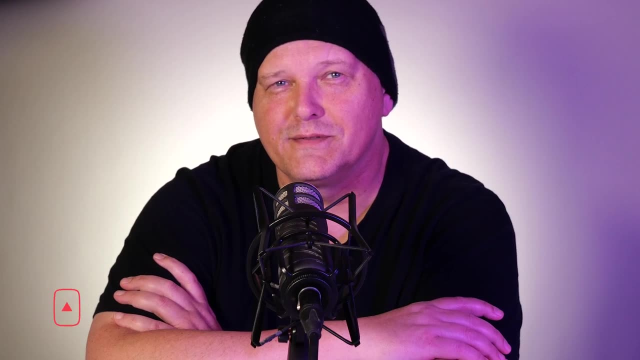 data, you're likely going to use DML. If you're creating objects like tables, you're likely going to use DDL. Thanks for watching. Don't forget to like and subscribe, and we'll see you soon. 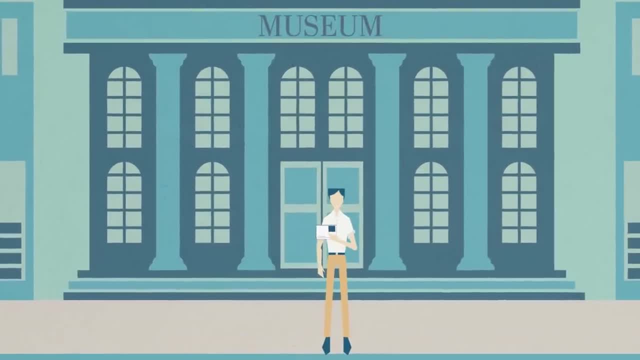 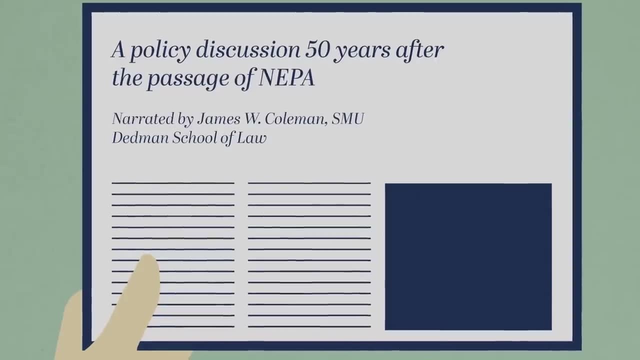 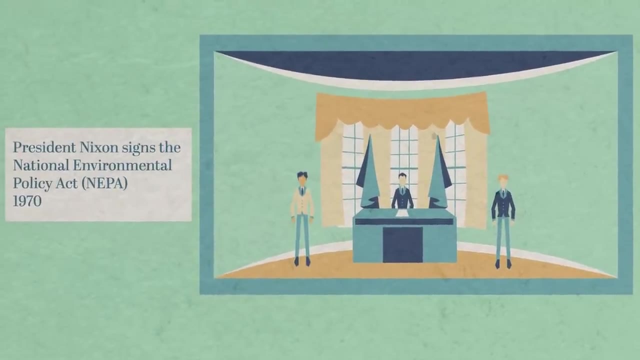 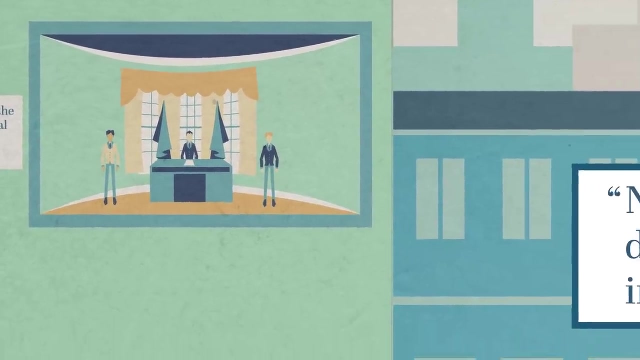 Does federal permitting under the National Environmental Policy Act need reform- A policy discussion 50 years after the passage of NEPA. 50 years ago, President Nixon signed the National Environmental Policy Act into law. The act requires the federal government to study the environmental consequences of new projects before it gives them a permit for construction. 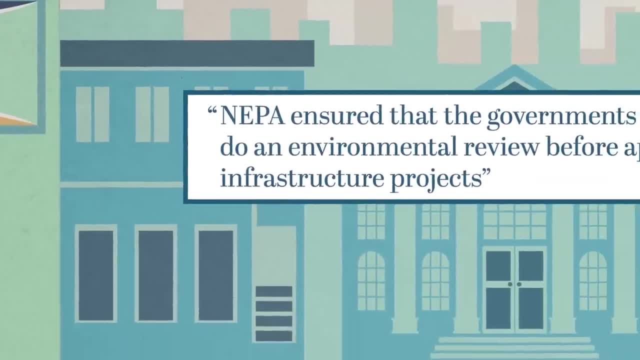 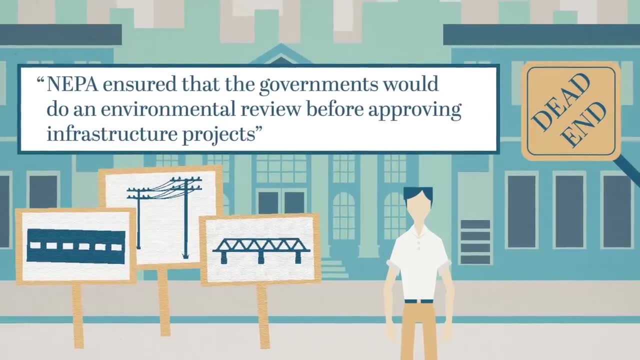 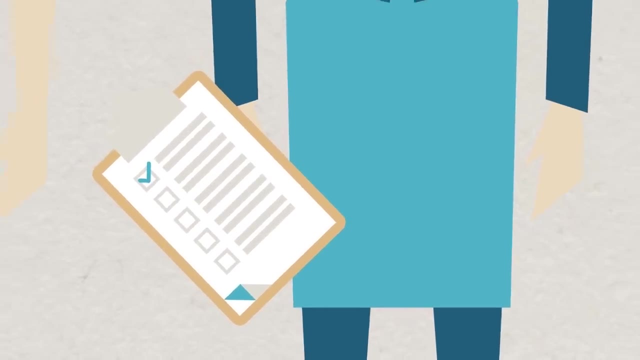 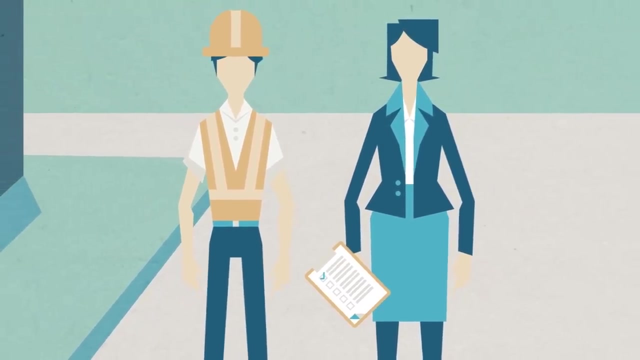 The National Environmental Policy Act, or NEPA, ensured that the governments would do an environmental review before approving infrastructure projects such as roads, pipelines and power lines. The government would take a few months to write a brief report describing and explaining the environmental impact of all the new projects it approved Over time. the NEPA review process. became much longer. NEPA requirements can be extremely costly For states, localities and private citizens who seek federal funds or permits, and for federal infrastructure projects. By 2008,, the average environmental review took three and a half years and was hundreds of pages in length. The result: Delay of critical infrastructure projects. 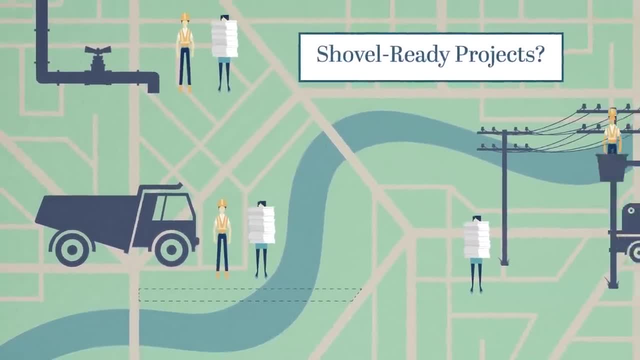 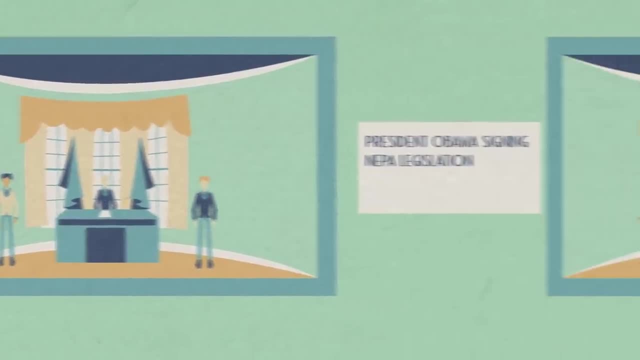 including President Obama's shovel-ready infrastructure proposals in the 2009 stimulus. Both President Bush and President Obama issued executive orders and signed the National Environmental Policy Act. The NEPA review process was time-consuming and the NEPA review process was too long to. 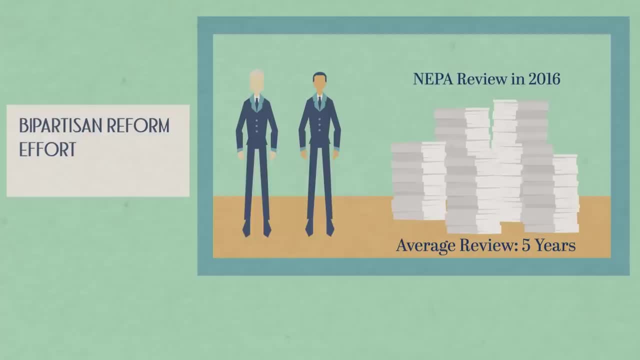 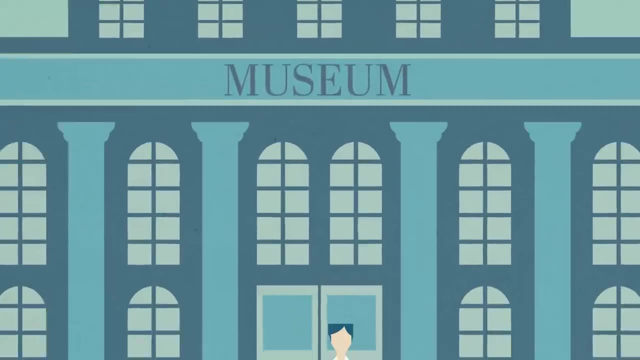 be reformed. The NEPA review process was too long to be reformed, But despite bipartisan reform efforts, these reviews keep getting longer. By 2016,, the average review took over five years, But since previous efforts to shorten NEPA reviews have 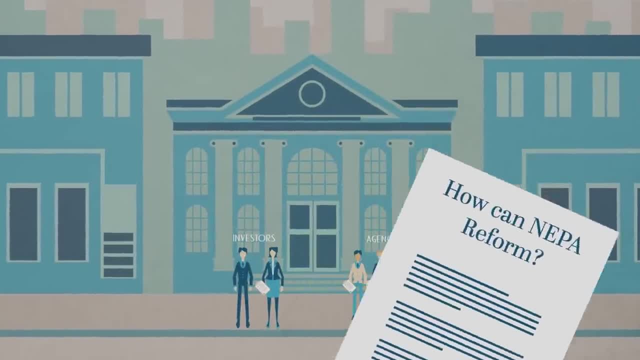 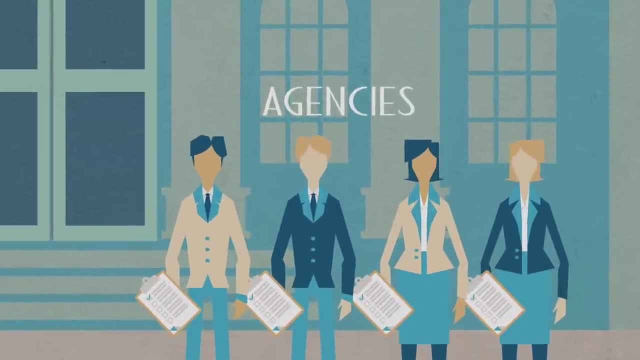 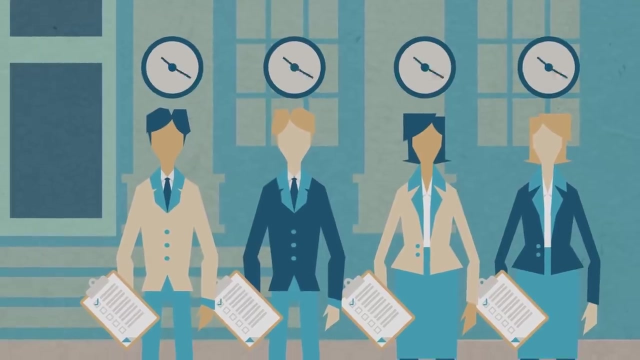 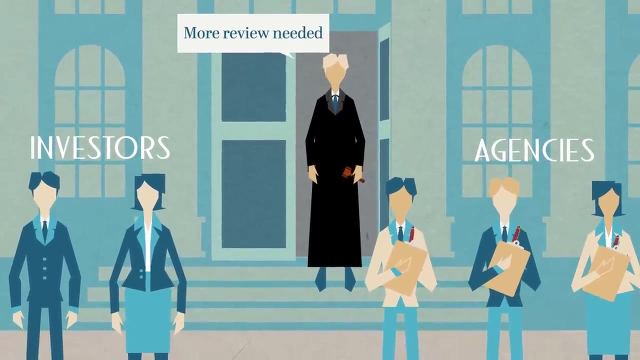 failed. how could it be reformed? Thus far, clarifying procedures and declaring faster timelines haven't been able to stop the drift toward longer reviews. Agencies are taking their time to try and survive judicial review. Federal courts keep demanding longer and longer reviews to comply with the National Environmental Policy Act.